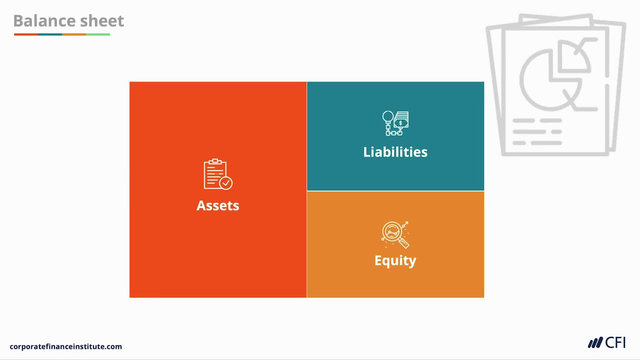 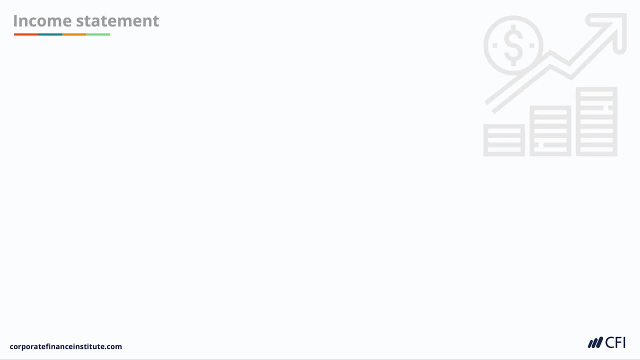 It contains the assets, liabilities and equity of a company. The balance sheet is an important component in determining the financial strength of a company. The income statement, also called the profit and loss statement or the statement of operations, contains the transactions of a company. 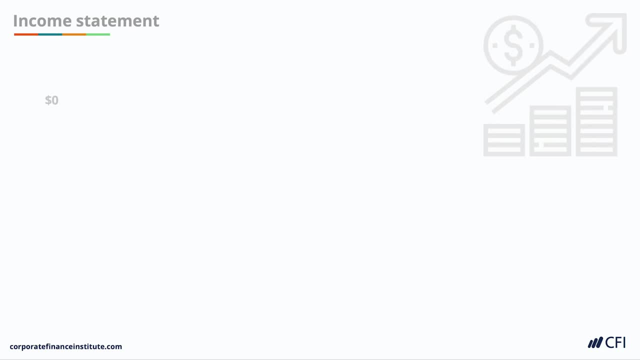 For a period of time. the income statement starts at a zero balance at the beginning of a fiscal year and records all of the transactions affecting revenues and expenses throughout the year. At the end of any period, it shows the amount of revenue earned, expenses incurred and. 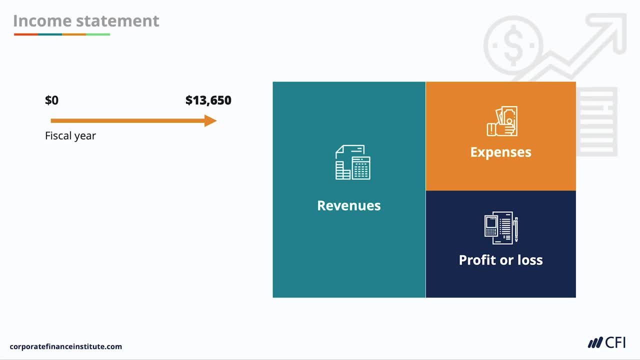 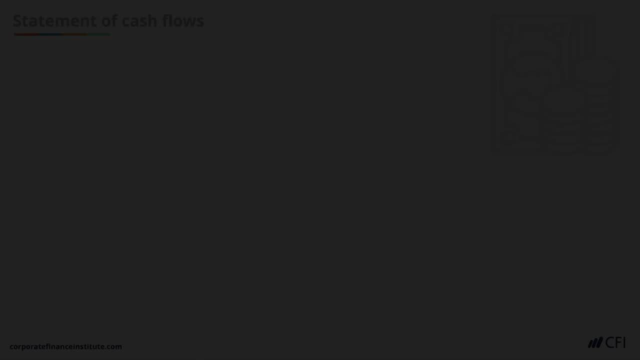 the net profit after amortization, interest and taxes are factored in. Therefore, the importance of the income statements is in showing the profitability of the company. The statement of cash flows- There are multiple different types of credit and loss statement as a kind of bank statement for a company. 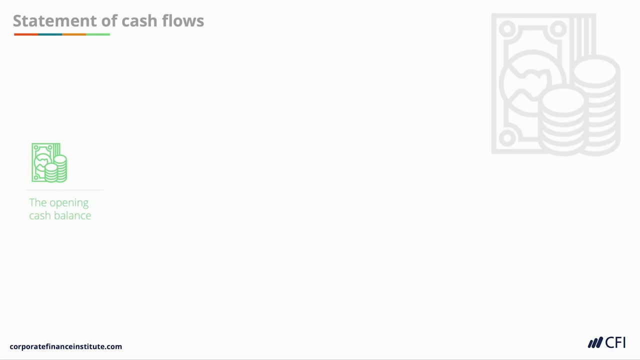 It shows the opening cash balance of the company and then lists all of the transactions affecting cash to arrive at the closing cash balance. The closing cash balance will match the balance reflected on the balance sheet. The difference between the bank statement and the statement of cash flows is that the 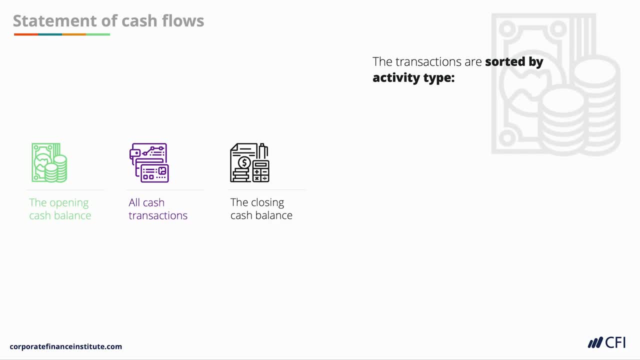 cash transactions are sorted by activity type. On the statement, cash flows are sorted by operating activities, investing activities and financing activities. The statement of cash flows, therefore, is a very useful financial statement to understand where cash is being generated and where it's being used in the business. 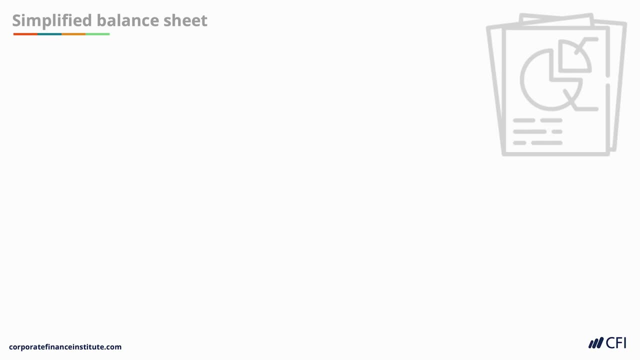 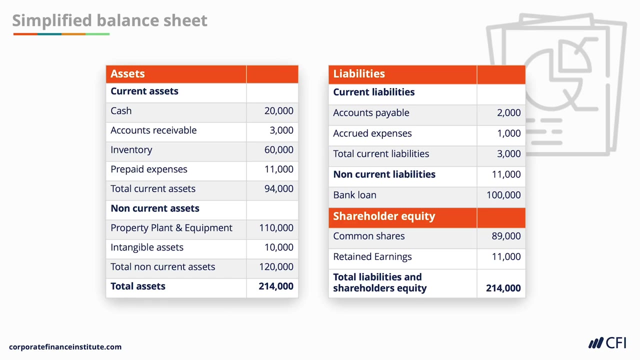 It's time to start exploring the balance sheet in more detail. Here is a simplified balance sheet that contains the most commonly used accounts. The balance sheet is presented in a horizontal format, with the assets on one side and the balancing, liabilities and equity showing on the other side. 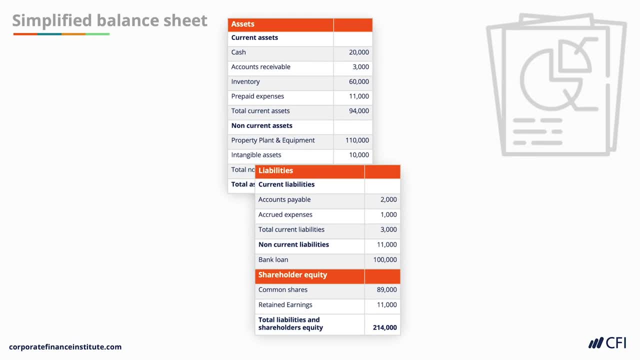 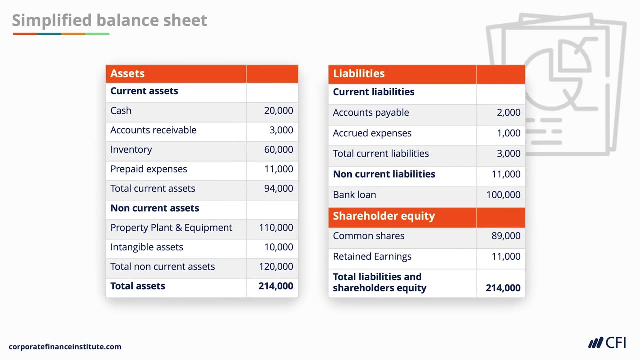 It's also commonly presented in a vertical format. The balance sheet represents the financial position or strength of the company. You can see that, based on the total assets versus total liabilities, this company appears to be financially stable. One item to explore further is the separation of assets and liabilities into current and 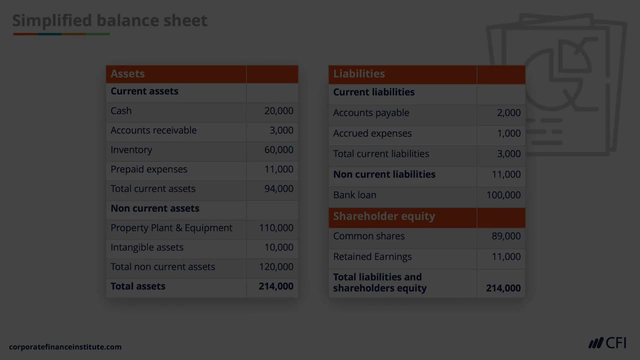 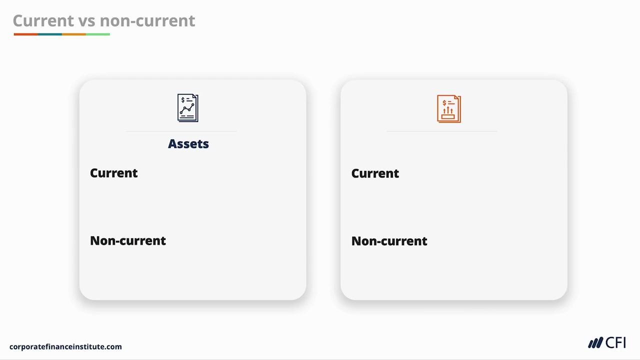 non-current items and the equity components. As you have seen, the balance sheet is separated into current and non-current sections on both the assets and liabilities sides of the balance sheet. Current assets are those that are expected to be converted into cash in less than a year. 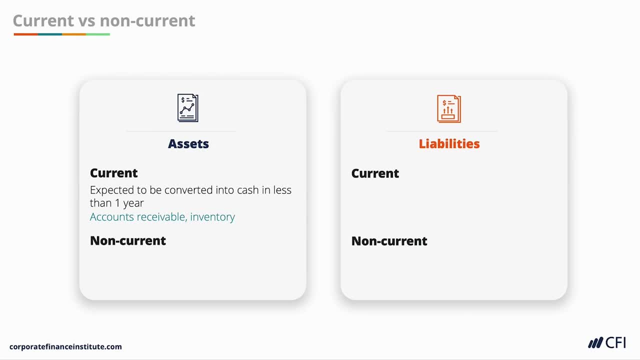 and include items like accounts, receivable and inventory. Non-current assets are those expected to be held for greater than one year and include items such as property, plant and equipment. The same holds true for current liabilities. These are liabilities that will be paid in less than a year. 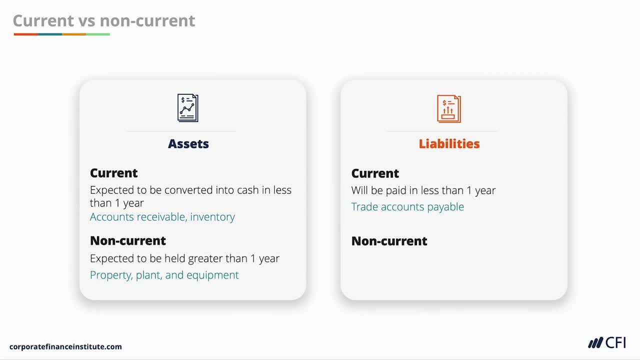 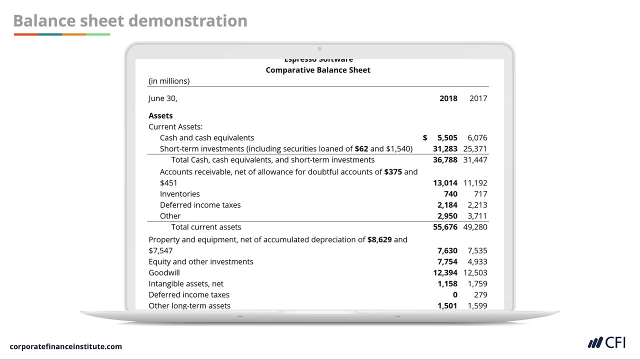 Trade accounts payable are a good example of a current liability. Non-current liabilities are those that have repayment terms that are longer than one year. An example would be a loan repayable over a five-year period. Let's look at Espresso Software's balance sheet as an example of what a typical reporting. 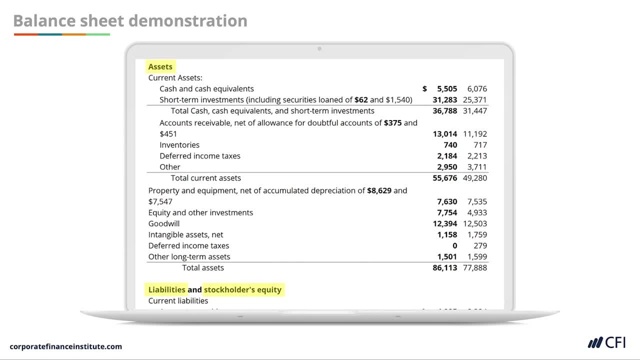 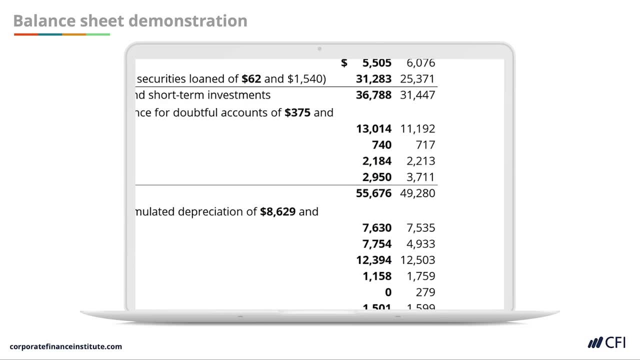 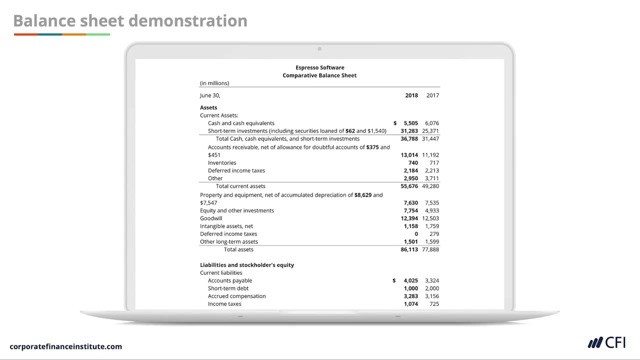 company will include for its assets, liabilities and equity. There are a few key items to note when you first look at the balance sheet. First, Espresso Software's statements are in millions of dollars. By reducing the numbers in this manner, the statements are a lot more readable. 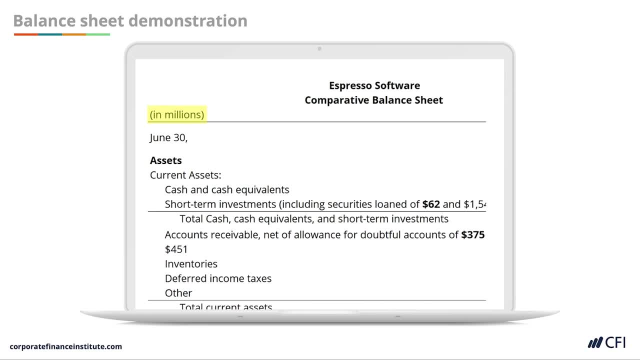 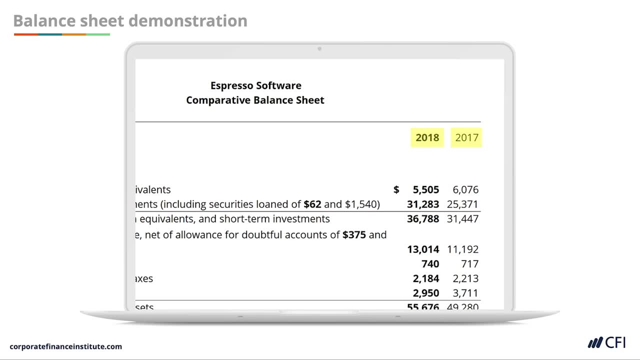 The statement will always have a notation. the numbers are not reported as whole dollars. Also, you'll see that both 2018 and 2017 accounts are reported. This is to provide the reader of the financial statement comparative results. You can compare this year to last year to see how the balances have changed. Finally, 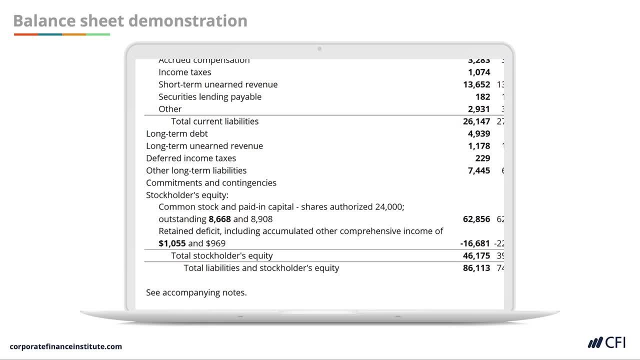 if you look at the bottom of the page, you will see the sentence: see accompanying notes. This is stated because the balance sheet on its own doesn't provide enough detail to allow the reader to understand what the company really owns and what it owes. We'll get to the financial statement notes a little later. 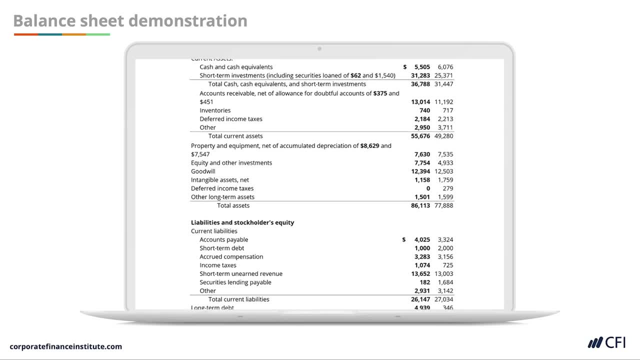 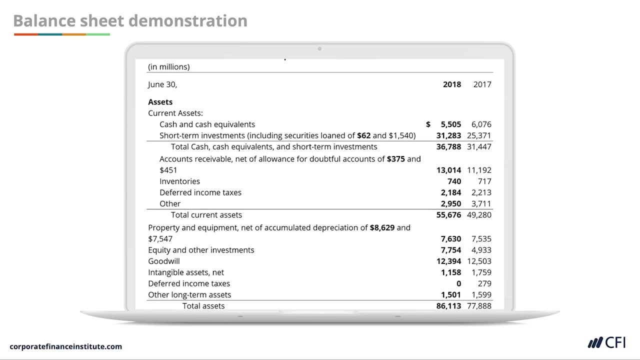 For now, let's spend some time focusing on the accounts making up the balance sheet. A lot of the balance sheet accounts should look familiar to you, For example, cash accounts, receivable, inventories, property, plant and equipment accounts payable. 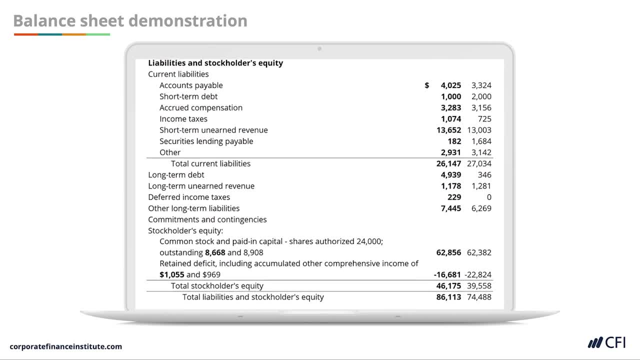 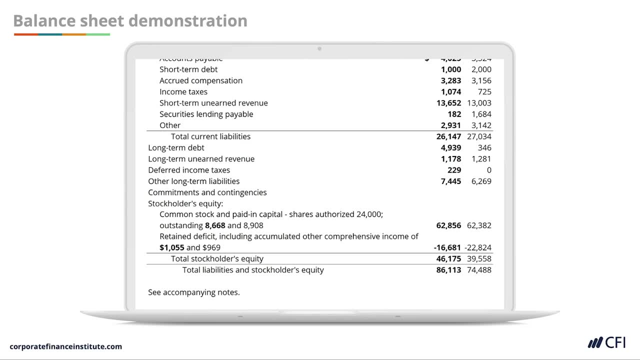 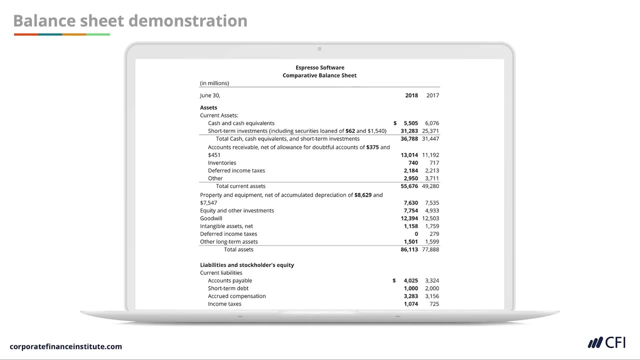 debt, common stock and retained earnings, Or, for Espresso software, retained deficit indicating that they've been accused, Or a company that's accumulating losses for a period of time. There are likely several balance sheet accounts that are unfamiliar to you. Let's take some time to explore those items in more detail. 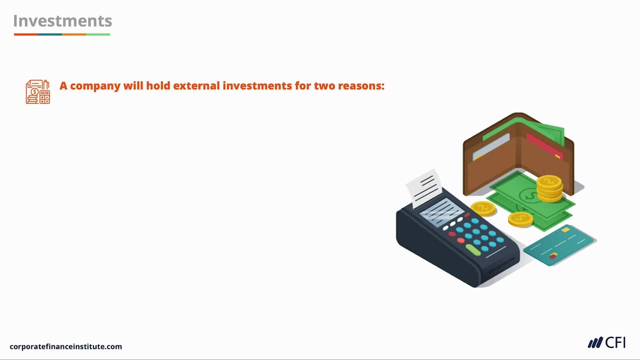 Oftentimes, a company will hold investments for two reasons. If it has excess cash that it doesn't have a use for within the very near term, or if it's accumulating it to make a large purchase, then it may make external investments. In this case, investments will be either short-term, where the investments will be held for less than 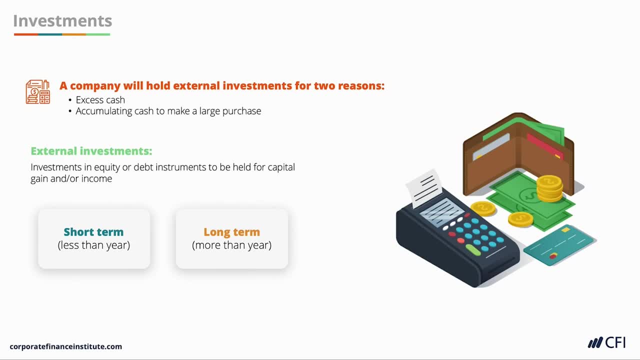 five years or less. If it's accumulated, it will be held for ten years or less, Or, if it's accumulated, a year or long-term, where they will be held for more than a year. The company may also make internal investments, for example in a joint venture or a subsidiary. 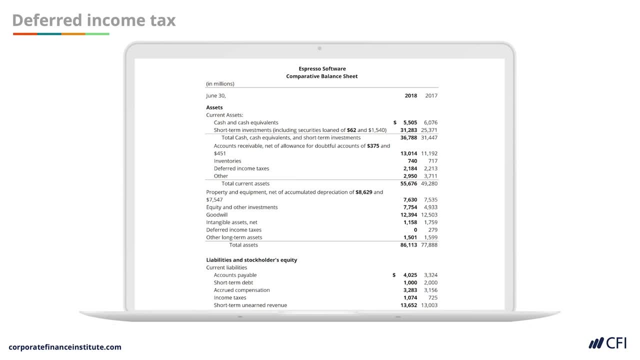 company Deferred income taxes are an item you will often see in financial statements For Espresso software. you'll see that they actually appear in several places on the balance sheet. They're found in the current and non-current asset sections, as well as in the non-current. 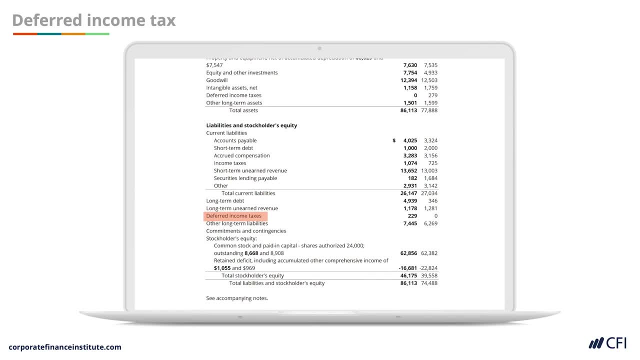 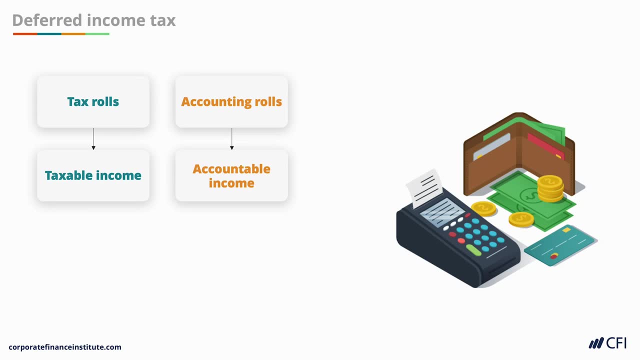 liability section. But what exactly are deferred taxes? The easiest way to explain them is related to tax rolls versus accounting rolls. When a company prepares an income tax return, they use tax rolls. These are not always the same as the accounting rolls. If the deduction is never allowed for tax purposes, then a permanent difference occurs. 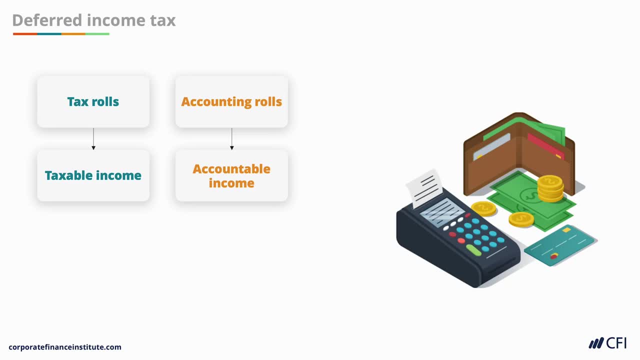 and no further work is required. However, if the deduction will be allowed in the future, then this is a timing difference and therefore recorded in the accounts. For example, depreciation or amortization on a piece of equipment might be calculated using the straight-line method for accounting purposes. 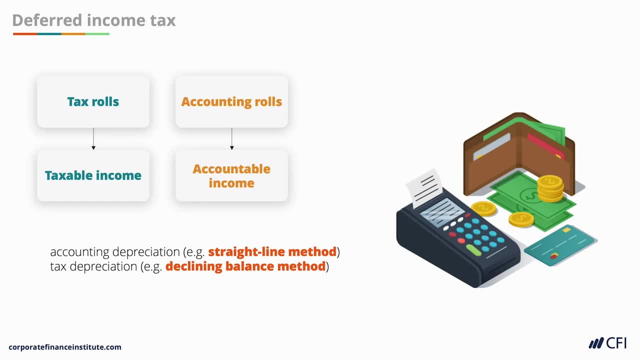 However, for tax purposes, an accelerated method is used. Therefore, the amount of taxes owing will be different until the equipment is fully depreciated. The difference between accounting income and taxable income is the basis for deferred income taxes, also known as future income taxes, and is recorded on the balance sheet. 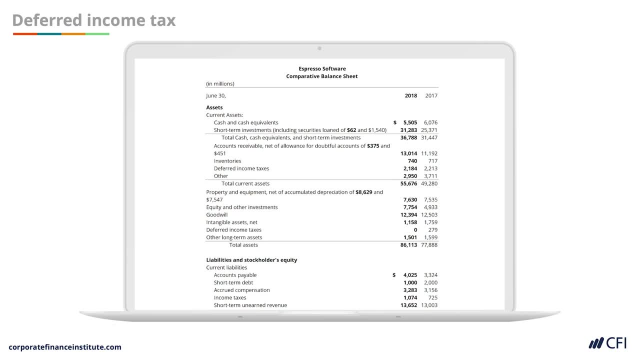 If there is less tax payable in the future, then the balance sheet is recorded on the balance sheet. If there is more tax payable in the future, it is an asset. If there will be more tax payable in the future, it is a liability. 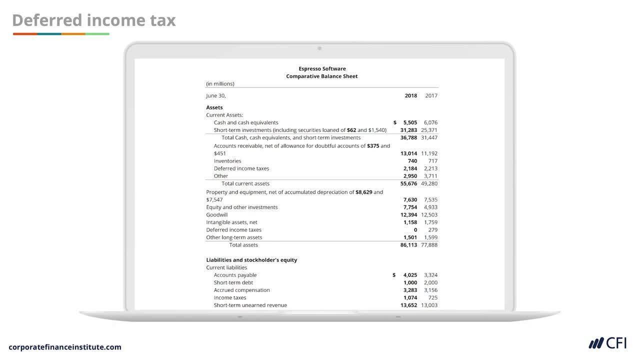 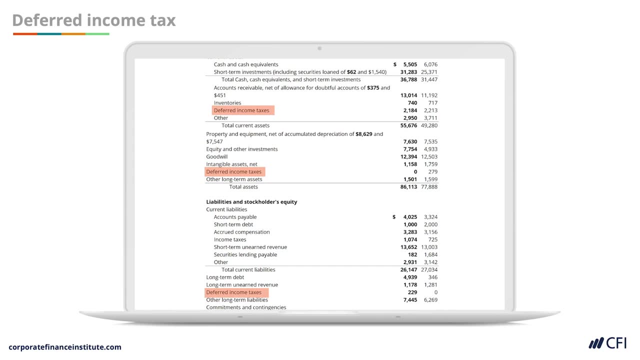 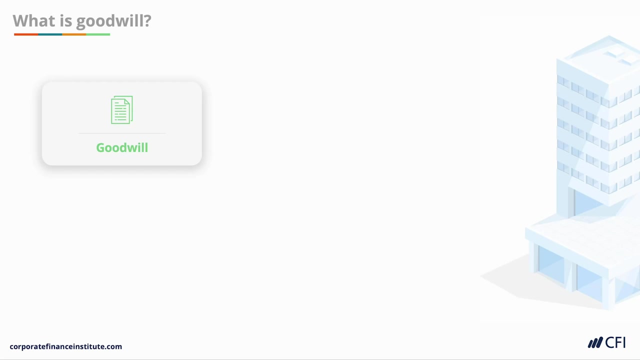 Accounting rolls don't allow the two amounts to be netted against each other. Therefore, if a company has timing differences going both ways, then both an asset and a liability will be recorded, much like we see for espresso software. Goodwill is another account seen in many financial statements. 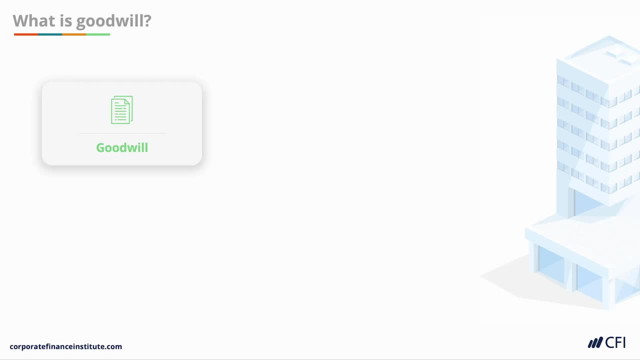 If a company has purchased for more than the fair value of its asset's less liabilities- which is also known as net assets- then the difference between the purchase price and the fair value is recorded as goodwill. It is considered an asset because the reason for paying more for a company's physical 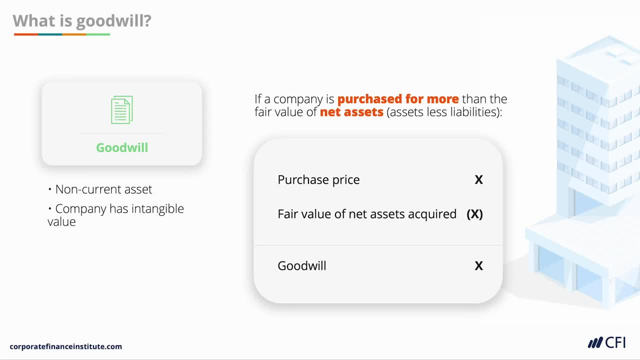 assets is because of the intangible value of the company. Things like brand, customers and intellectual capital are factored in. These factors are considered to be benefits that will last longer than one year, and hence why goodwill is recorded as non-current. 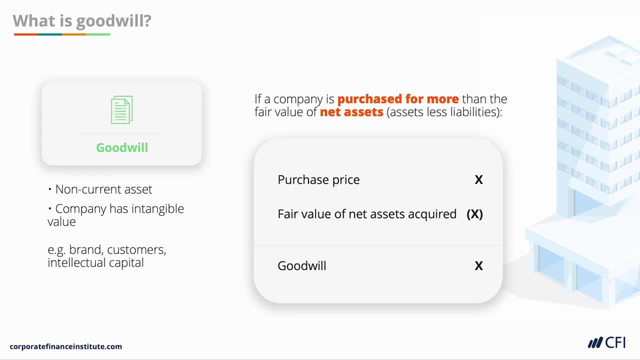 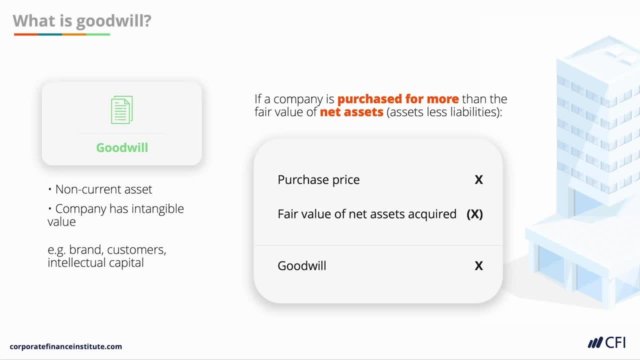 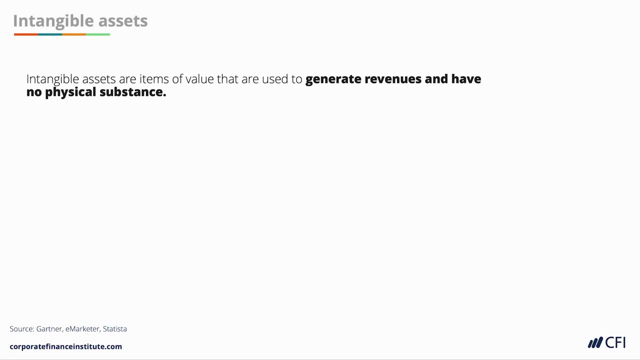 If not, it's written down to the amount considered to be fair value. Similar to goodwill, intangible assets are items of value that are used to generate revenue and have no physical substance. Examples would be the Coca-Cola trademark design or the Nike swoosh. 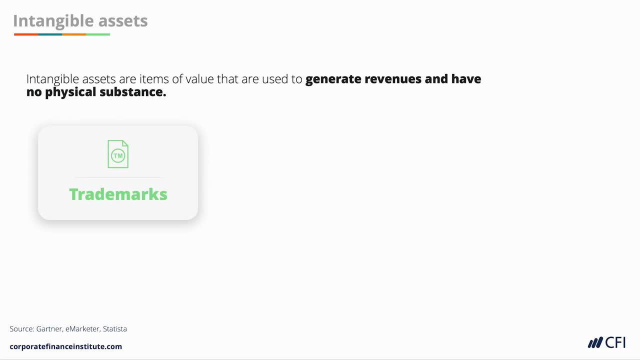 These trademarks have a value to the organization, are owned and cannot be used by others, and they enhance the earning potential of the organization. A patent to produce an innovative product had a cost to develop and apply for and will result in future earnings, so those costs are considered the cost to develop or purchase. 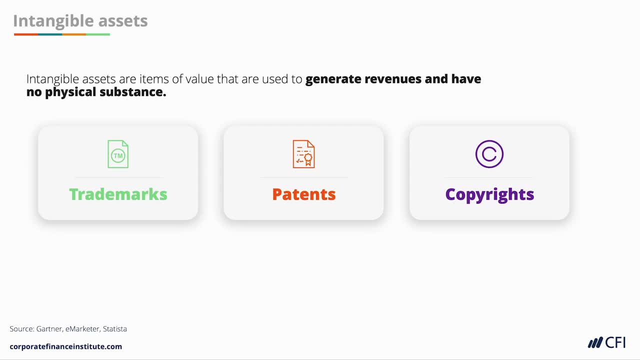 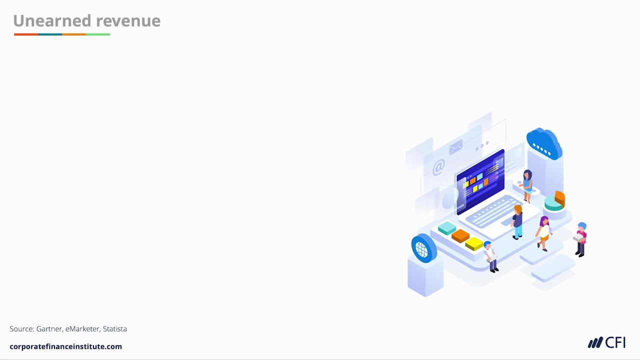 the intangible asset. Intangible assets appear on the balance sheet in the non-current section. They're amortized, much like physical assets are Unearned. revenue arises when a company sells something it has not yet delivered. In Espresso Software's case it's for software licenses and subscriptions over a period of 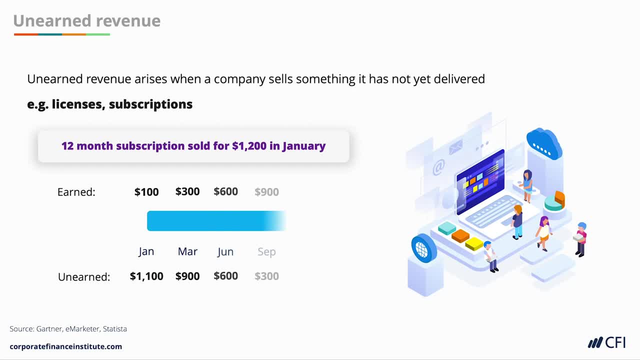 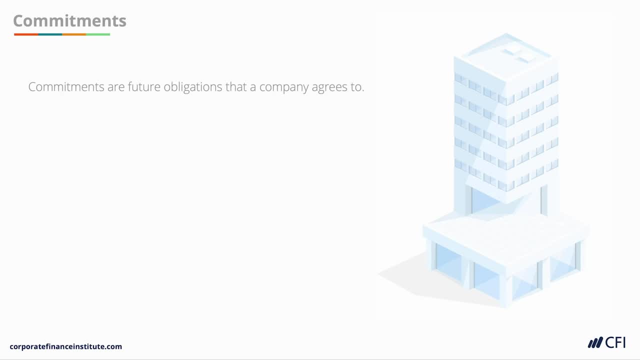 time. As the period expires, a portion of the subscription amount is included in income. The balance is shown as a liability. Commitments are future obligations that a company has agreed to. They're future liabilities for the company and therefore are disclosed in the balance. 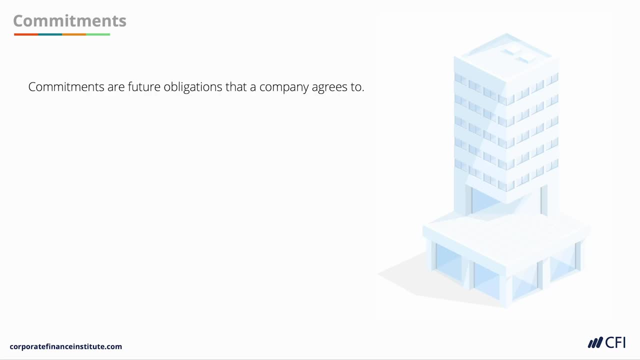 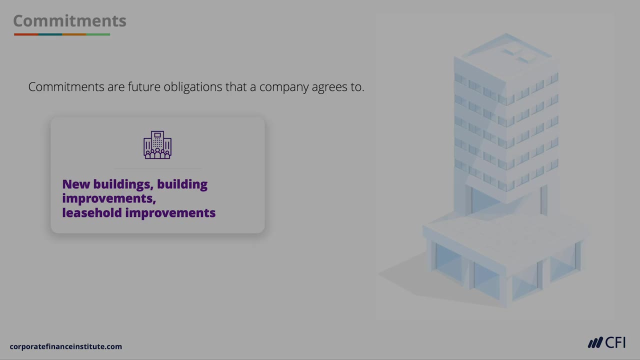 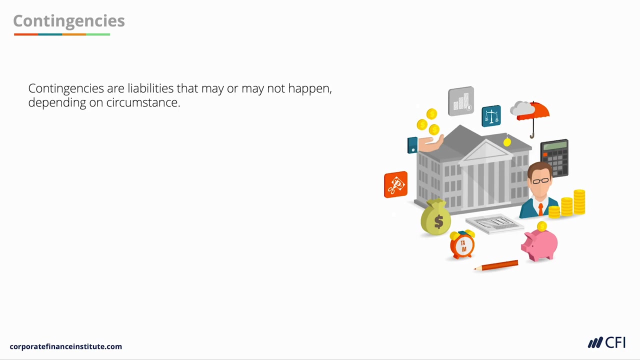 sheet so a reader is informed of the liability For Espresso Software. they've committed to constructing new buildings, building a plant and climbing three speaker towers to include bothitti. humanity Contingencies are things that may or may not happen, depending on certain circumstances. 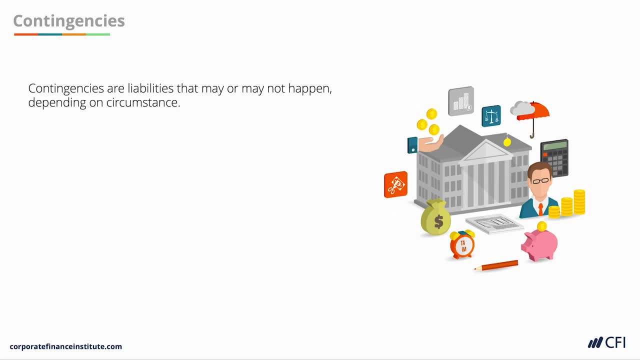 Readers of financial statements would want to know if there was likely to be a circumstance that could result in the company being liable. When it's likely a loss will suffer in the future and the amount can be reasonably estimated, then the contingent liability must be recorded on the balance sheet. 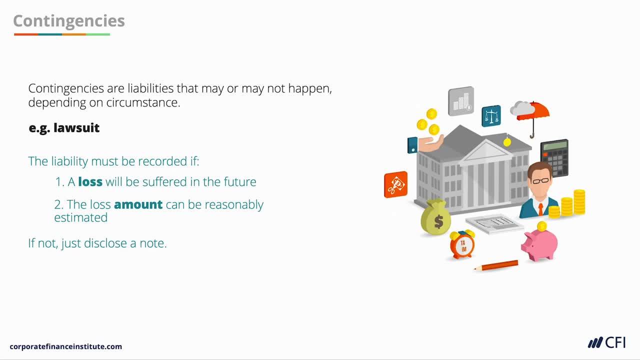 An example of a contingency, for example, would be the final settlement of a debate. You would spend a semblance of minutes upon antecedents on the account to solve the dispute With. the deed is decided at any time. The contention is quitewww well-played at the beginning. 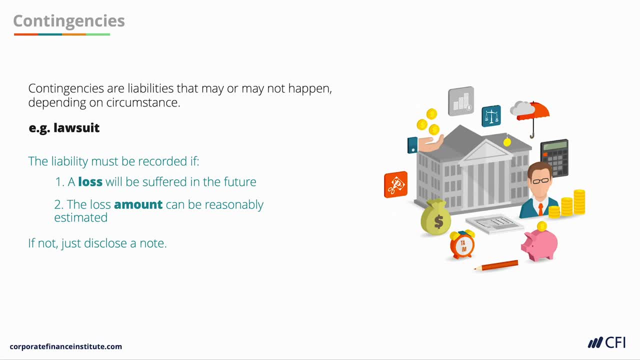 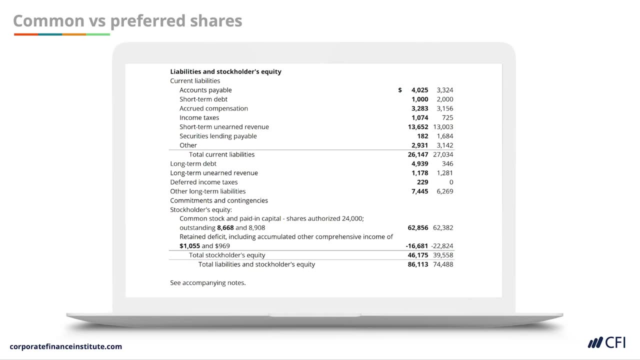 a company. if the company believes it will be unsuccessful and can estimate the amount it would have to pay, then it would set the amount up as a liability. under the shareholders or stockholders equity section of the balance sheet are where the shares of the company can be found. equity is almost always made up of. 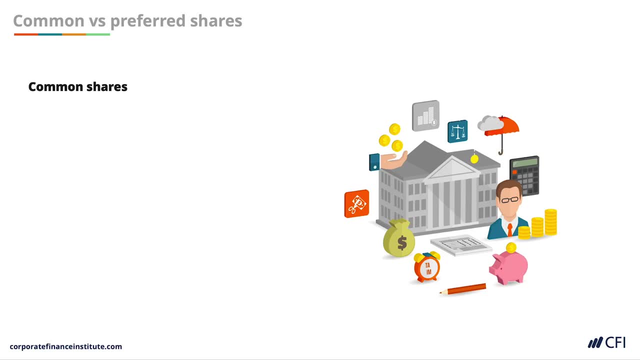 common shares, also known as common stock. common shares allow for participation in the profits of the company. after all, debtors and preferred shareholders are paid. the participation normally comes in the form of a dividend. common shares also allow for voting rights in a company. common shareholders are usually 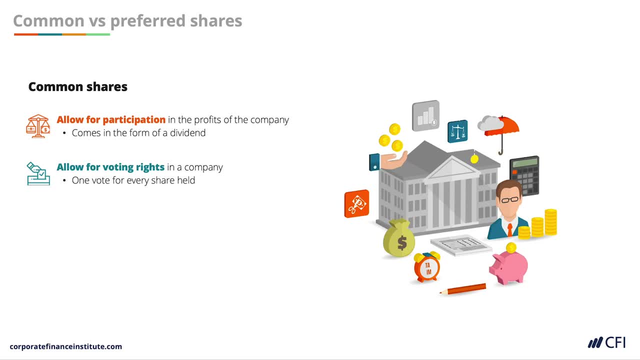 allowed to cast one vote for every share held. finally, if a company were to be dissolved, any residual amount after everyone else was paid would go to the common shareholders. equity may include preferred shares, preferred shares or preferred stock. you are different than common shares in the way that shareholders participate. usually, 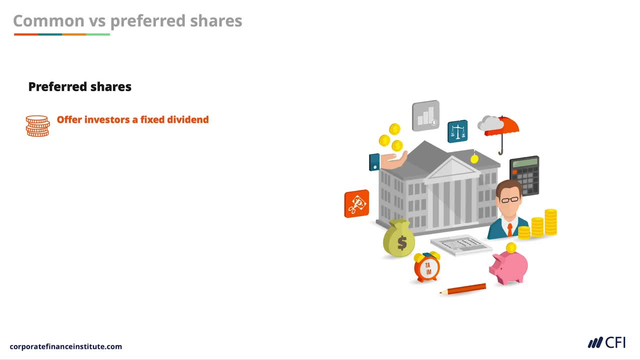 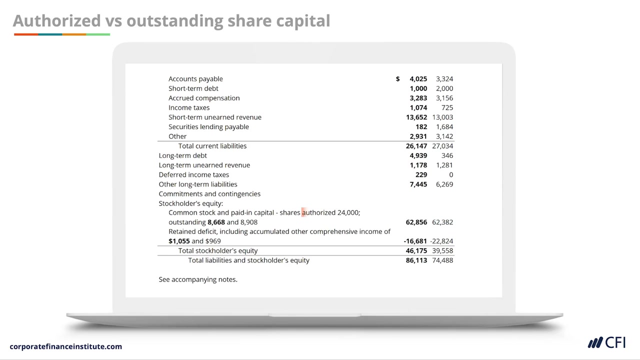 preferred shares offer a fixed dividend. however, the dividend may not be paid annually. preferred share dividends will accumulate and be paid before common share dividends are paid. a balance sheet normally indicates shares authorized and those outstanding, but what's the difference? authorized shares are the total number of shares. 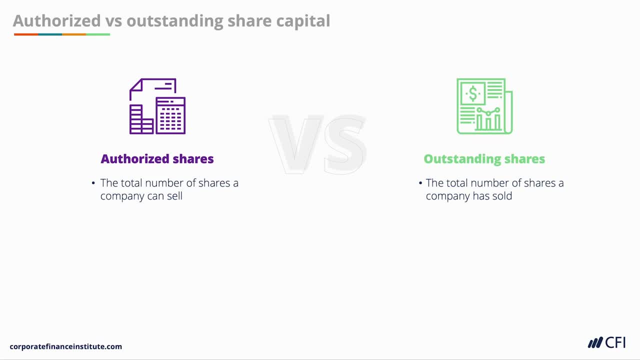 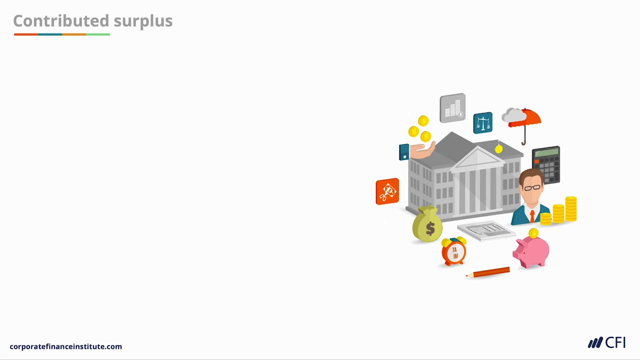 that a company has to sell outstanding shares are the total number of shares the company has sold. • natural contrast •. actually, the balance sheet may also show outstanding shares as issued or paid out shares. one final item that may appear in the equity section of a company's balance: 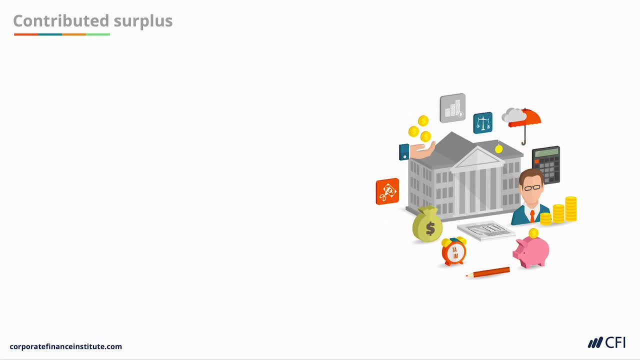 sheet is contributed surplus. a company may issue shares with a par value. par value is simply the face value of the share on issuance. where a company receives more for the share than its par or face value, then the excess amount is referred to as contributed surplus. 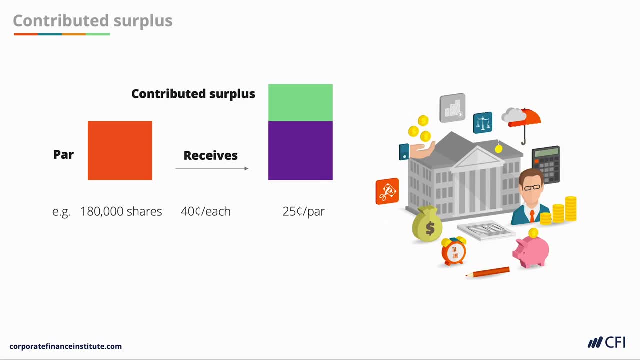 Let's look at a simple example. If a company were to issue 180,000 shares for 40 cents each and shares have a par value of 25 cents, how would this be shown on their balance sheet? There'd be two lines. The first would be the paid-up or paid-in share capital of 180,000. 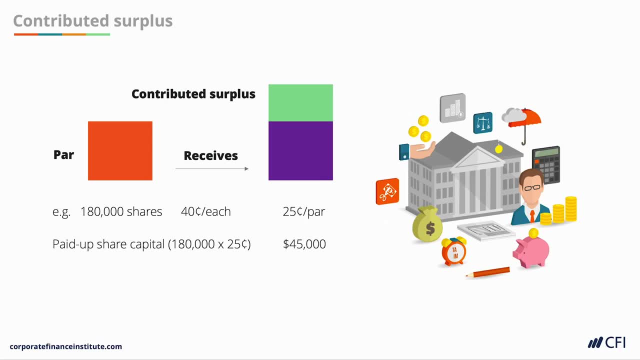 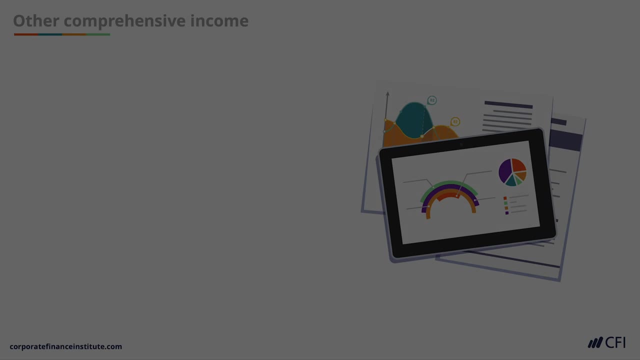 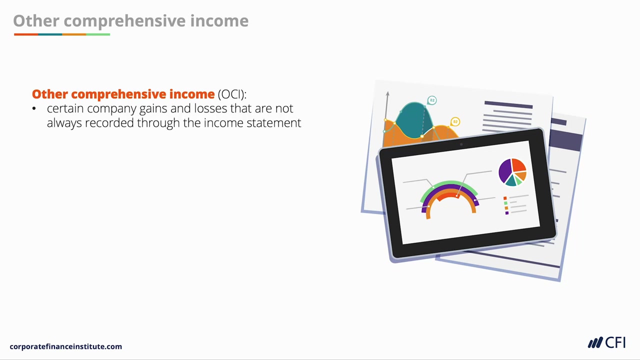 multiplied by the 25-cent face value, for a total amount of $45,000.. The second would be contributed surplus for the difference of 15 cents, multiplied by the 180,000 shares, for a total of $27,000.. Other Comprehensive Income, or OCI, represents certain gains and losses that a company may have. 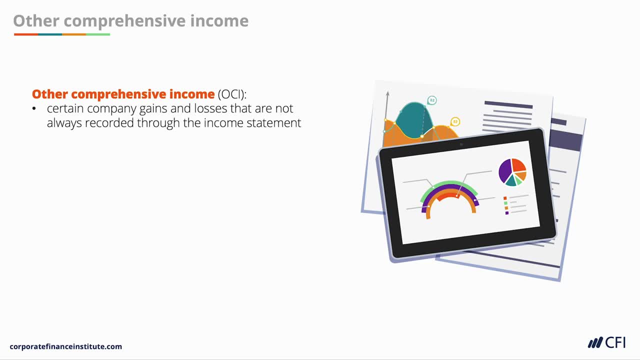 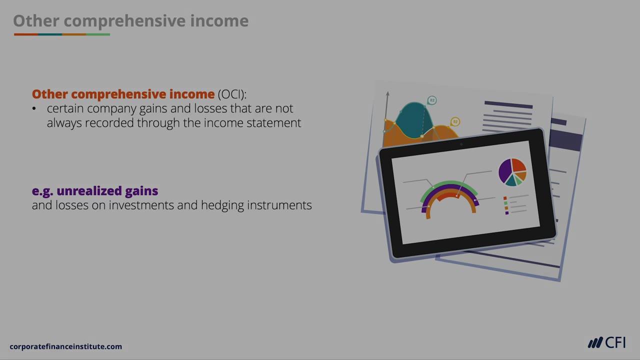 that are not always recorded through the income statement. Instead, they go directly to Retain You Earnings. Examples of typical items within OCI include unrealized gains and losses on investments and hedging instruments. OCI is recorded in the equity side of the balance sheet, Sometimes the statement of shareholders'. 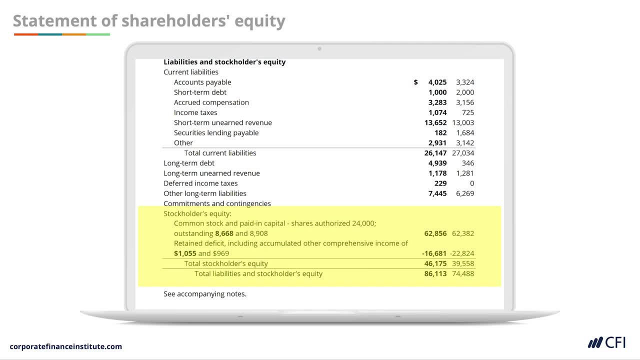 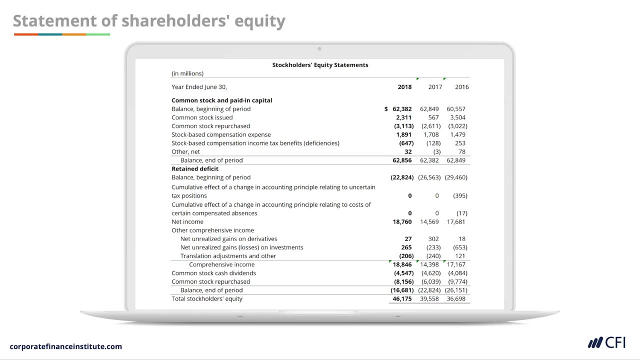 equity will show at the bottom of a company's balance sheet. Other times it will show as a separate financial statement. The statement of shareholders' equity is made up of all the equity transactions for the year. It's usually broken into components. One component: 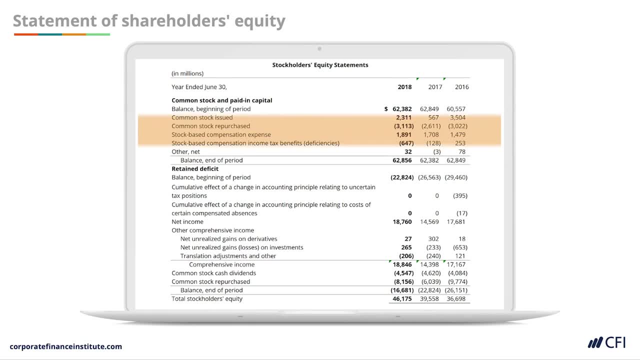 shows all of the share or stock transactions that occurred during that year. The other component is related to retained earnings and all of the transactions affecting it for the year. The statement starts with the opening balance of each component, shows the activity for each and then ends with the component's closing balances. 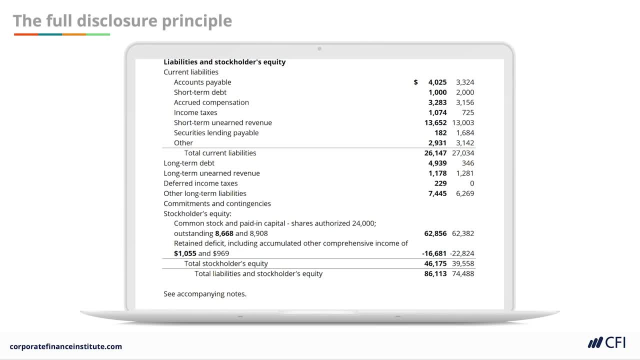 A critical part of reading a set of financial statements relate to the notes that accompany them. Take, for example, Espresso Software's balance sheet. Without the notes of the financial statements, do you know how inventory is recorded, what's included in deferred income taxes or what commitments the company has made? The actual financial 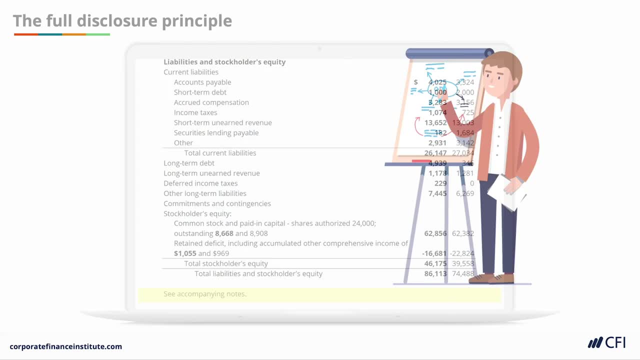 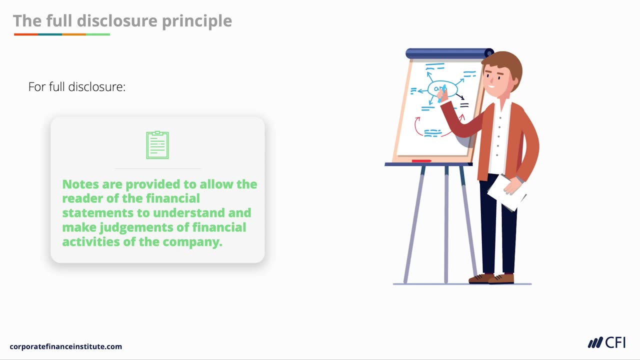 statements themselves only tell part of the story. In order to provide full disclosure, notes are provided to allow the reader of the financial statement to understand and make judgments of the financial activities of the company. There are three types of notes of the financial statements. 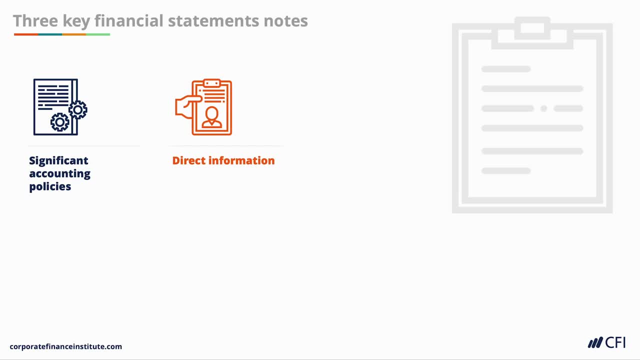 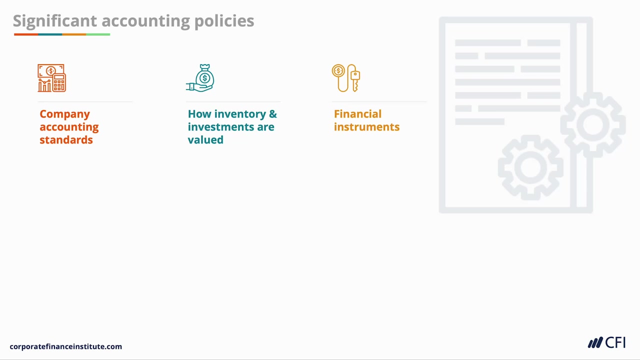 Significant accounting policies, direct information and indirect information. Perhaps the most important financial statement note is the first one that's presented: the significant accounting policies note. This note presents important information such as which accounting standards the company follows, how inventory and investments are valued, what type of financial instruments the company has, how revenue is.